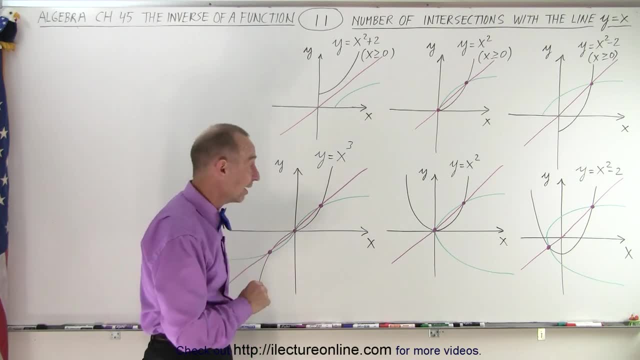 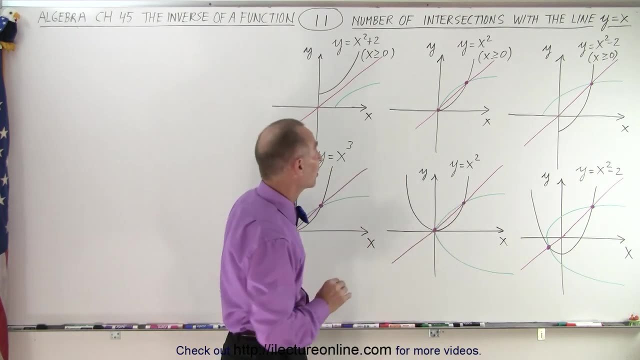 Now what is interesting is that: where did it cross the y equals x line? Well, it turns out they crossed the y equals x line at the very same point, And that's a very unique concept right here. Take a look at there. 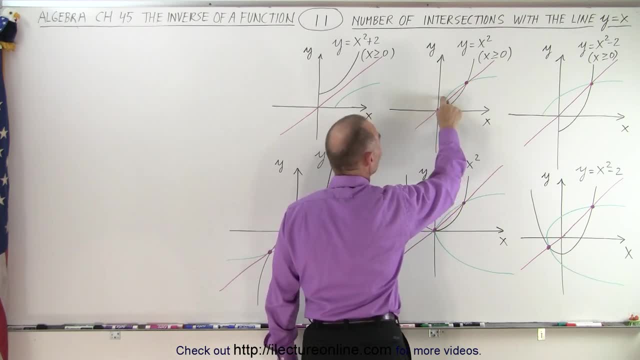 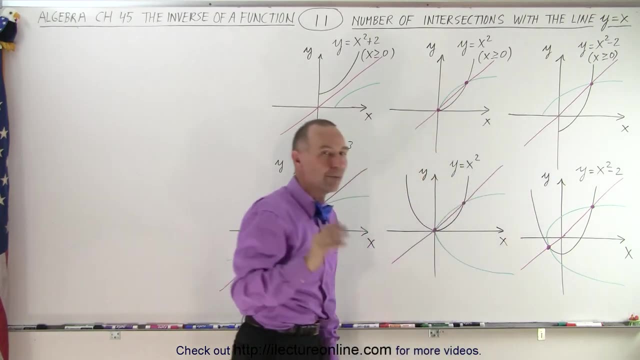 You see that right here they crossed this point, both of the inverse of the function and the function itself. Here again, the inverse of the function, the function itself. Wherever the line is crossed, both the function and the inverse of the function cross that y equals x line at the very same place. 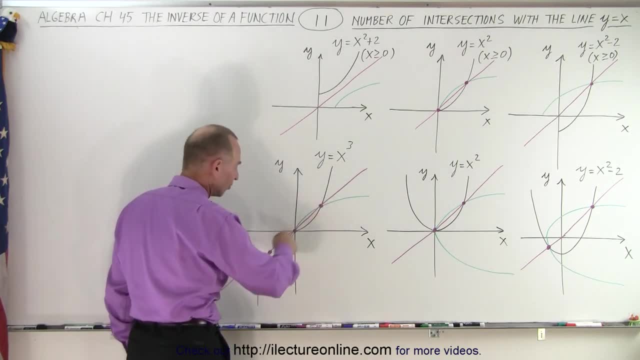 And notice over. here we have the function y equals x cubed. It's an odd function And notice that the inverse of the function crosses the y equals x line at the very same locations as the function itself crosses, And this case is three crossings because of y equals x cubed. 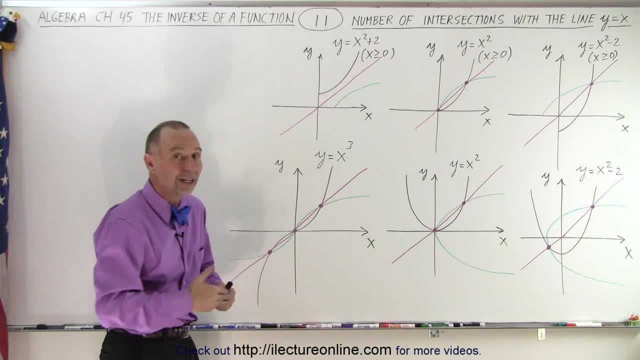 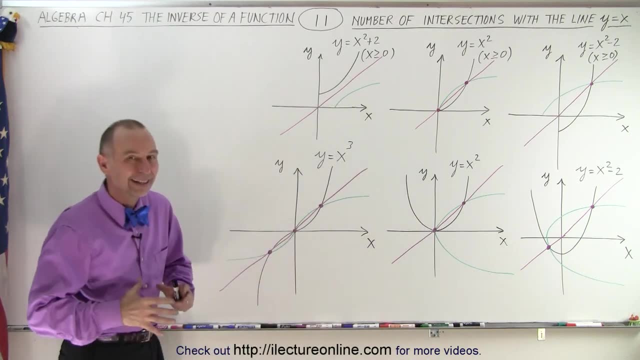 Now it doesn't always mean that there's going to be three crossings, But it can be as many as three crossings when we have y equals x cubed, versus only two crossings when we have y equals x squared- At least the max number of crossings. 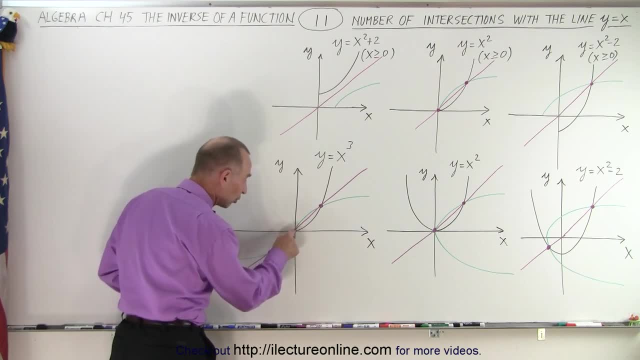 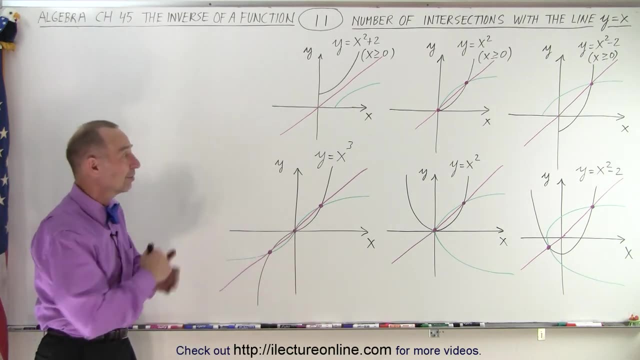 But at any rate, notice that both the function and its inverse will cross the y equals x line at the very same location each and every single time, And that is what we know about the inverse of function relative to the function, the way it relates to that y equals x line. 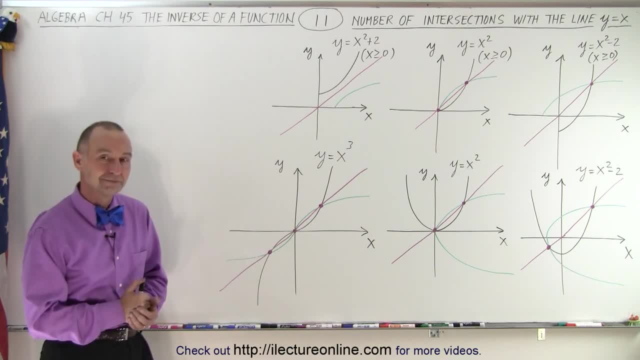 And that is how it's done. Does it mean anything? Well, it means that they cross the line at the same place. It makes it easier to graph- right, It makes it easier to graph And it does give you a little bit more insight into that mirror image concept. 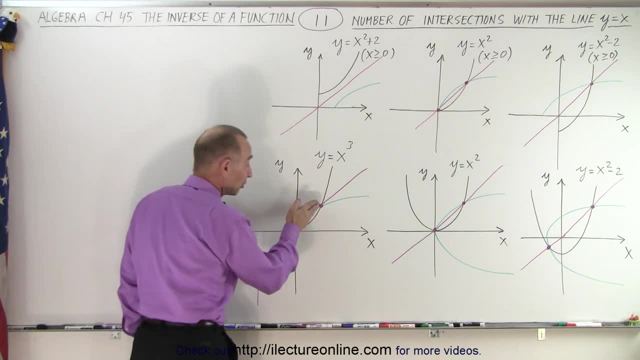 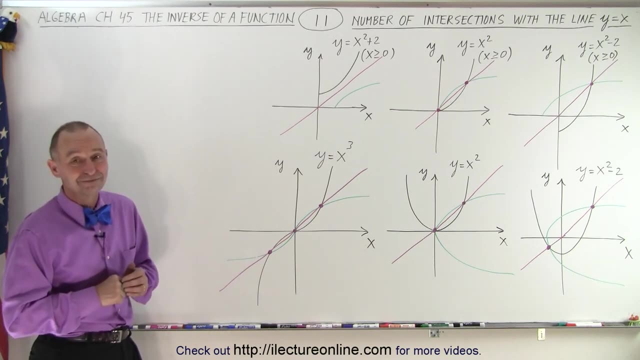 Because the reason why they do that is because there is a mirror image. Whenever one crosses, the other one has to cross, Otherwise you don't have the mirror image, And that's, in essence, the significance of that Now, but is there anything that you will use it for, say in physics, chemistry or biology? 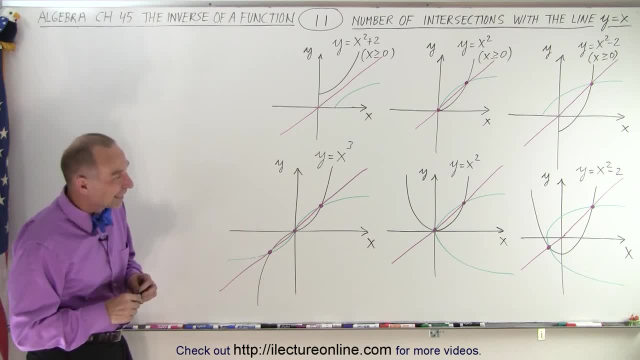 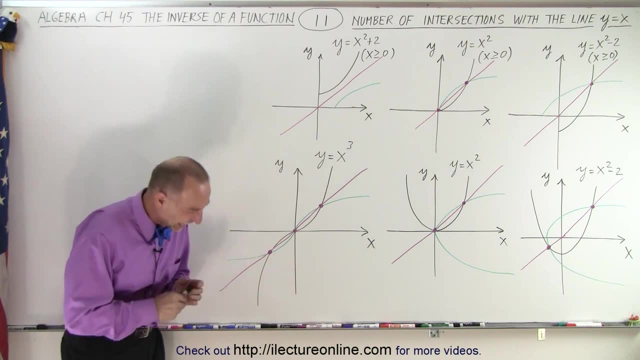 Like factor of growth or chemical mixtures, decaying velocity and acceleration intersecting something. There are actually probably because I can't be 100% sure, but if I think what you just mentioned, there are places where the concept of the function and its inverse do have a special meaning.